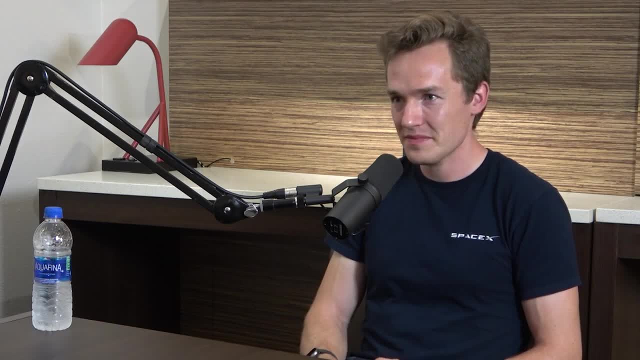 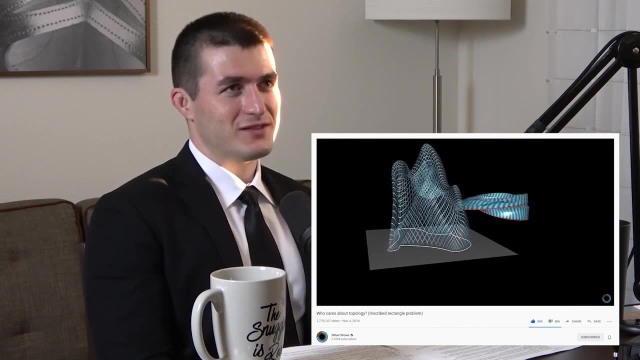 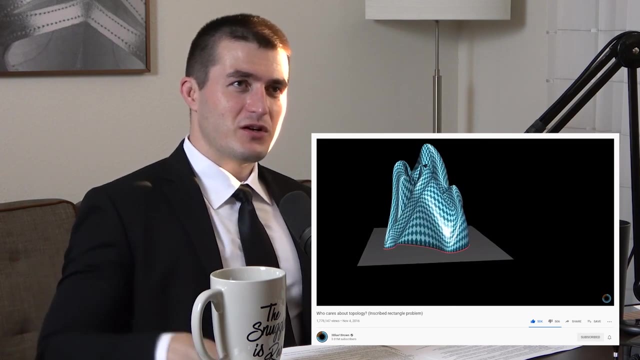 further. it would take more time, And one of your cooler videos, the homomorphic like from the Mobius strip to this. What do you describe? rectangle? Yeah, That's a super. and you're like, yeah, you can't. you can't transform the Mobius strip into a, into a surface. 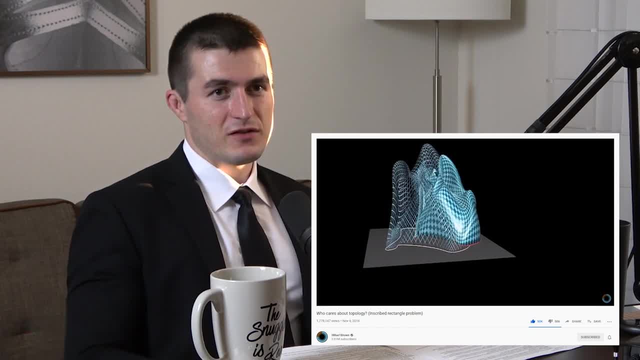 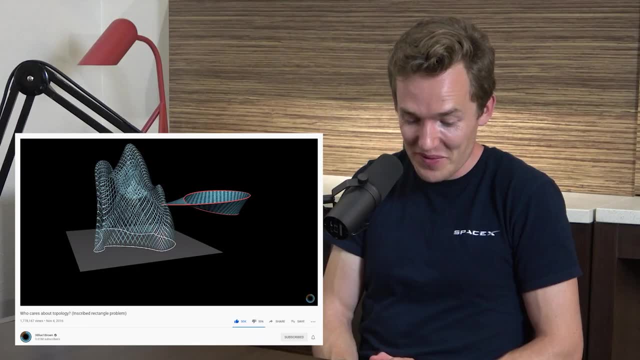 without it intersecting itself. But I'll leave it to you to to see why that is. Well, I hope that's not exactly how I phrase it, Cause I think what, what my hope would be is that I leave it to you to think about why you would expect that to be true. 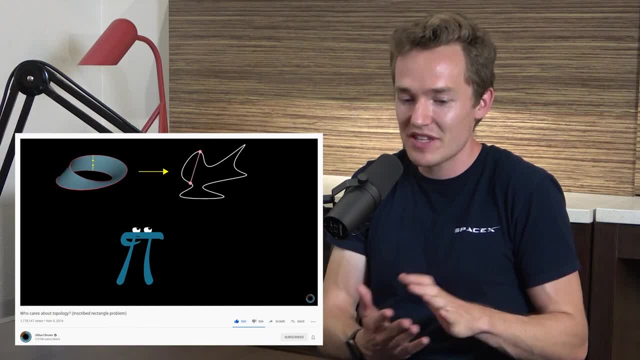 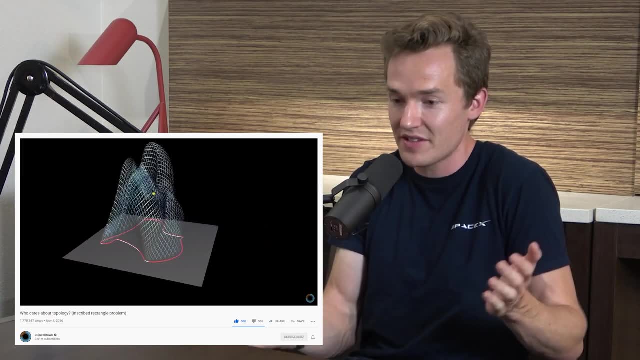 And then to want to know what aspects of a Mobius strip do you want to formalize such that you can prove that intuition that you have Cause at some point now you're starting to invent algebraic topology. If you have these vague instincts like I, want to get this Mobius strip, I want to 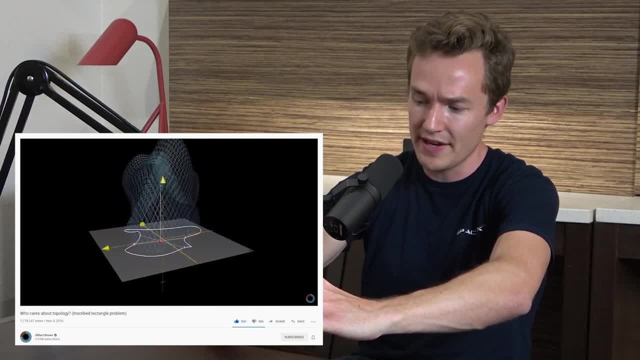 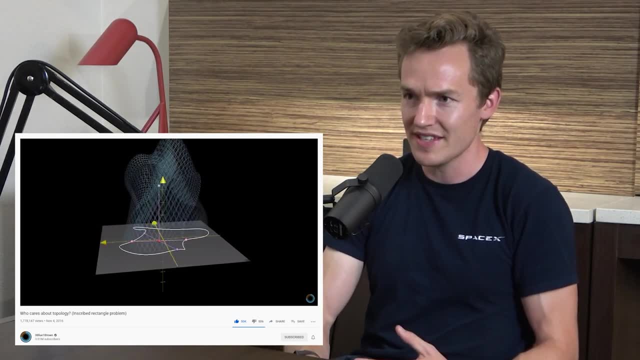 fit it such that it's all above the plane but its boundary sits exactly on the plane. I don't think I can do that without crossing itself, but that's that feels really vague. How do I formalize it? And as you're starting to formalize that, 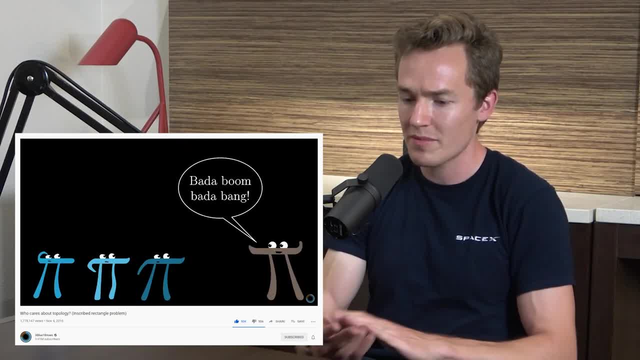 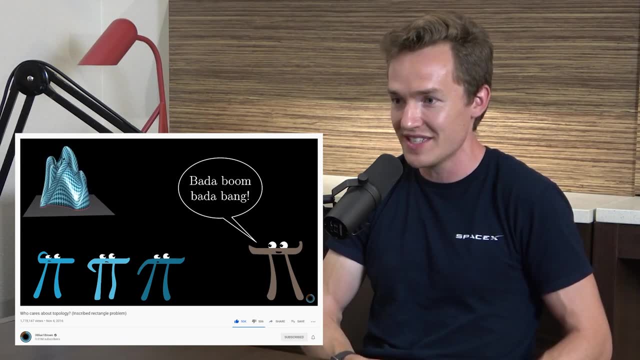 that's what's going to get you to try to come up with a definition for what it means to be orientable or non-orientable And like, once you have that motivation, a lot of the otherwise arbitrary things that are sitting at the very beginning of a topology stack textbook start to. 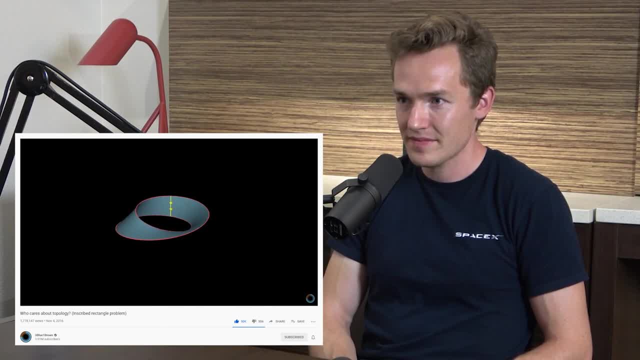 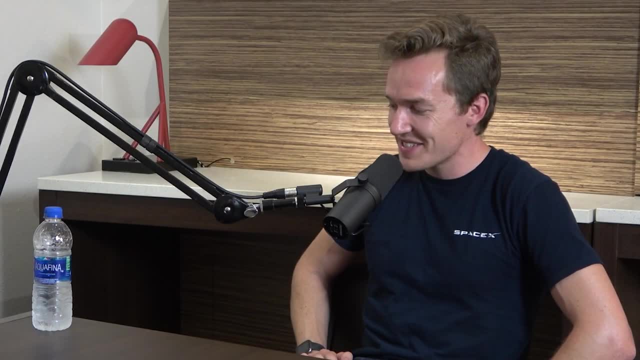 make a little more sense. Yeah, And I mean that that whole video beautifully was a motivation for topology is cool. That was my. well, my hope with that is: I feel like topology is um, I don't want to say it's taught wrong, but I do think sometimes it's popularized in the wrong way. 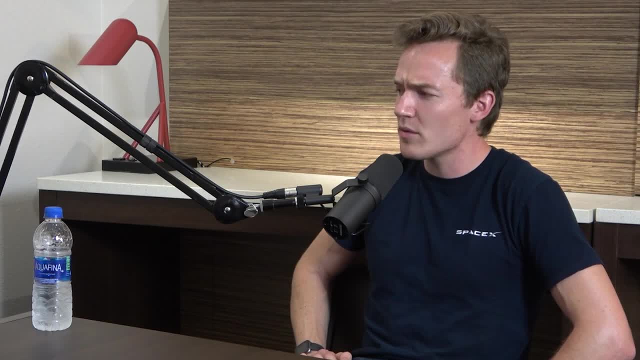 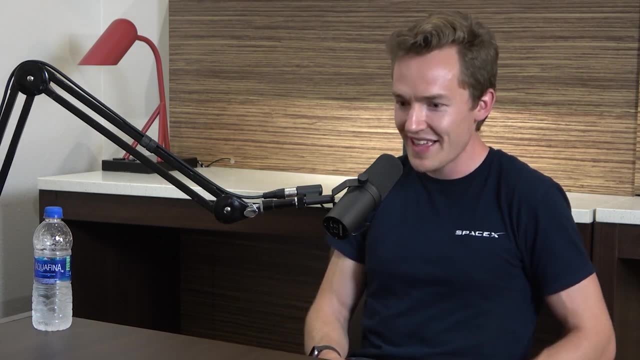 Where, uh, you know, you'll hear these things, with people saying: Oh, topologists, they're very interested in surfaces that you can bend and stretch, but you can't cut or glue, Are they Why? Yeah, There's all sorts of things you can be interested in with random. 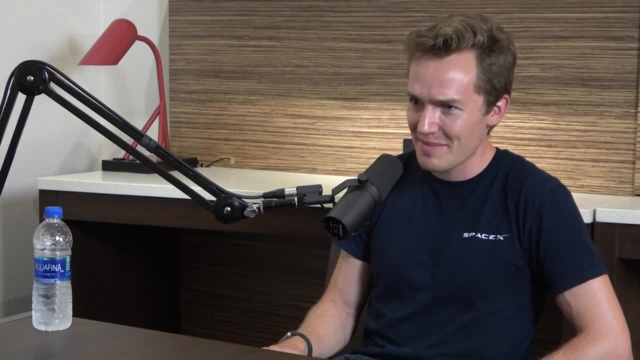 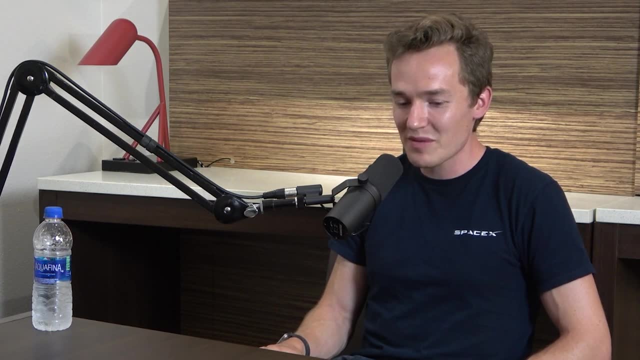 like imaginative, uh, manipulations of things. Is that really what like mathematicians are into? And the short answer is not. not really. That's uh. it's not. as if someone was sitting there thinking like: I wonder what the properties of clay are. I had some arbitrary rules about what. 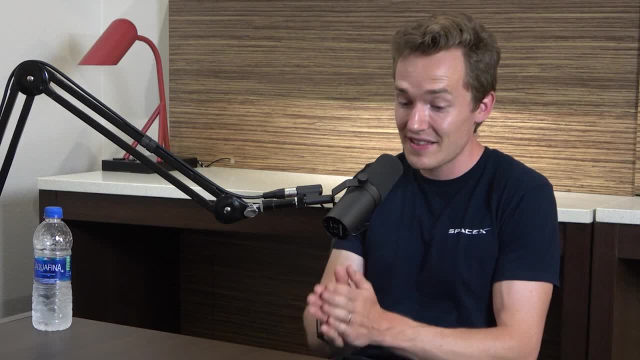 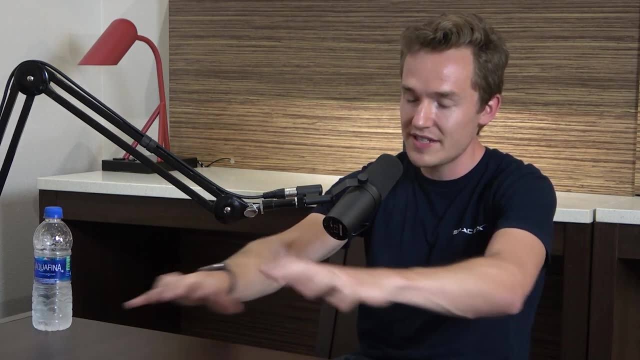 when I can't cut it And when I can't glue it. instead it's. there's a ton of pieces of math that um can actually be equivalent to, uh, like these very general structures. That's like geometry, except you don't have exact distances, You just want to maintain. 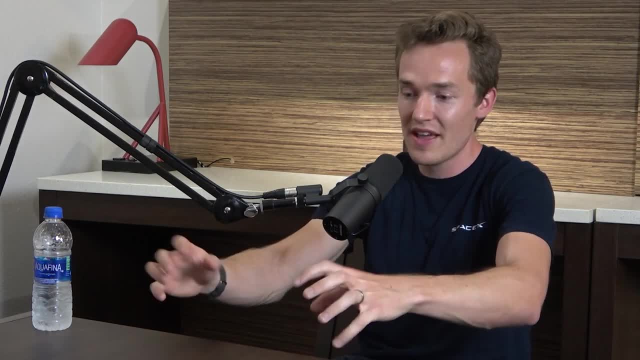 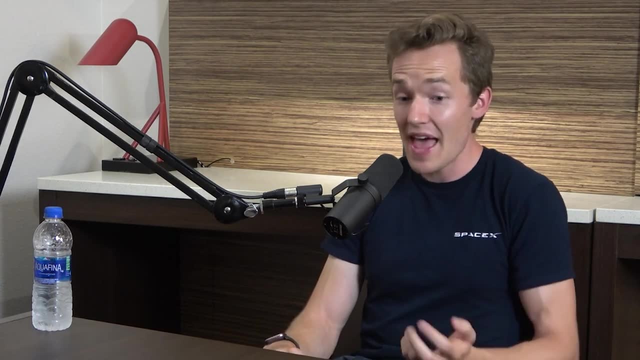 a notion of closeness And once you get it to those general structures, constructing mappings between them, translate into non-trivial facts about other parts of math And that I just I don't think that's actually like popularized Um, I don't even think it's emphasized. 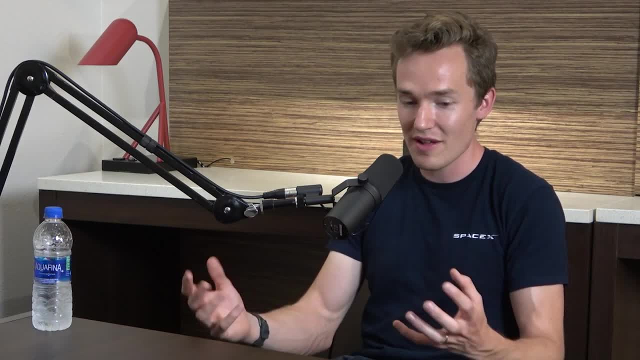 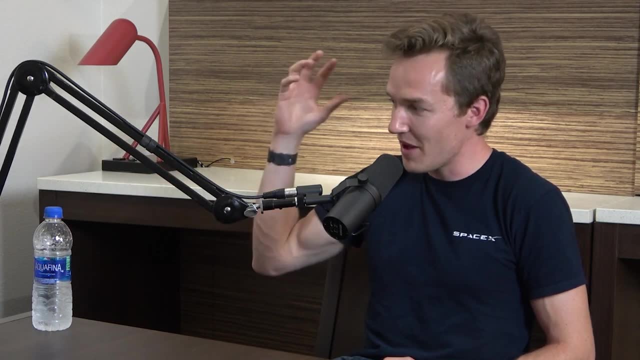 well enough, when you're starting to take a topology class cause, you kind of have these two problems. It's like either it's too squishy- You're just talking about coffee mugs and donuts- or it's a little bit too rigor first And you're talking about um, the axiom systems with open. 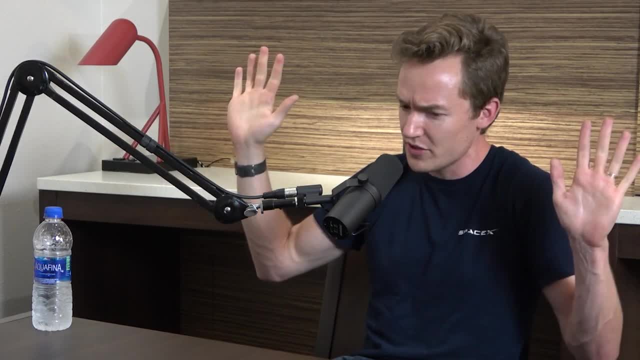 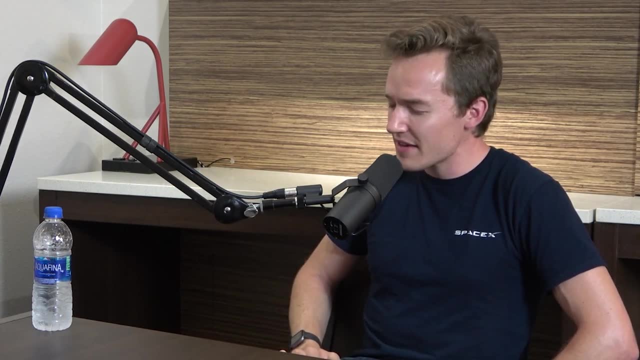 sets, and an open set is not the opposite of closed set. So sorry about that, Everyone. we have a notion of cloping sets for ones that are both at the same time. Um and just, it's not. it's not an intuitive axiom system in comparison to other fields of math. So you as the student, 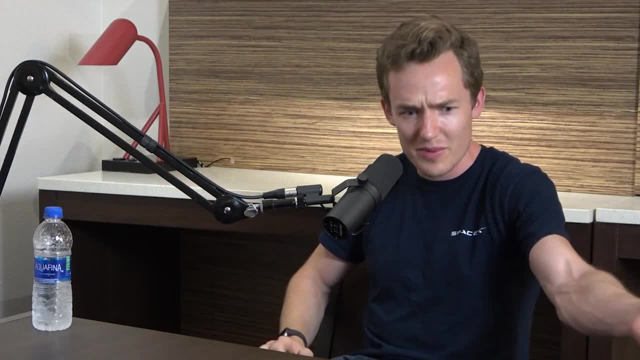 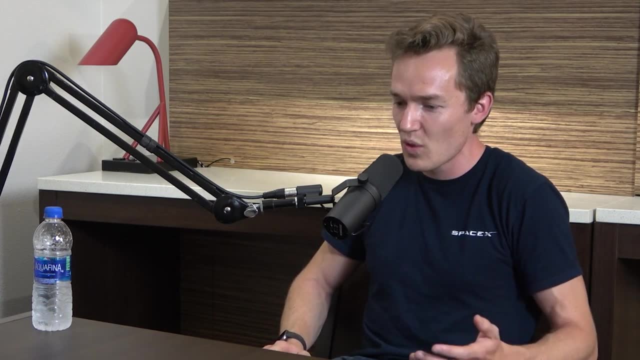 really have to walk through mud to to get there And you're constantly confused about how this relates to the beautiful things about coffee mugs and Mobius strips and such, And it takes a really long time to actually see math, like see topology in the way that mathematicians see topology. But I don't. 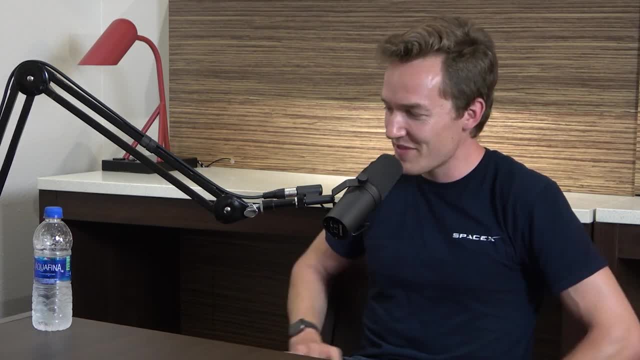 think it needs to take that time. I think there's um. this is making me feel like I need to make more videos on the topic, Cause I think I've only done two. Uh, but you know, I've also seen it in. 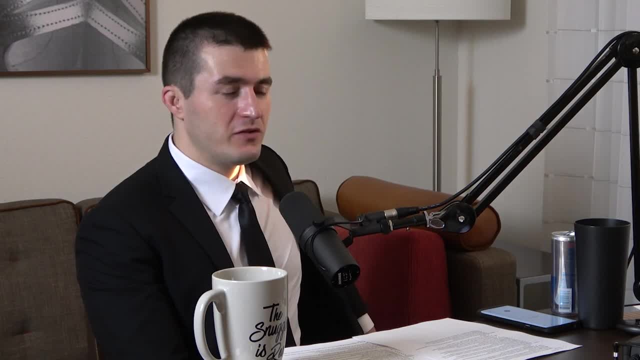 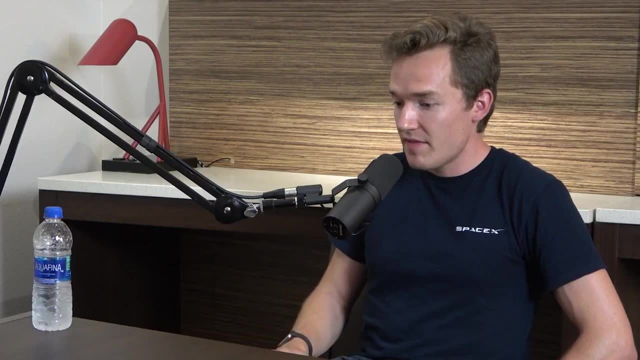 my narrow view of uh like, um, I'd find game theory very beautiful And I know topology has been used uh elegantly To prove things in game theory. Yeah, You have like facts that seem very strange. Like I could tell you, you stir your coffee and 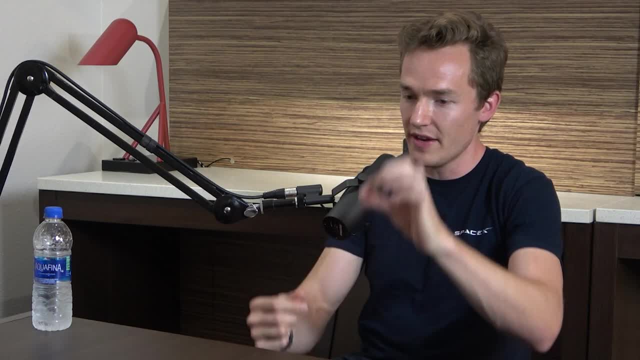 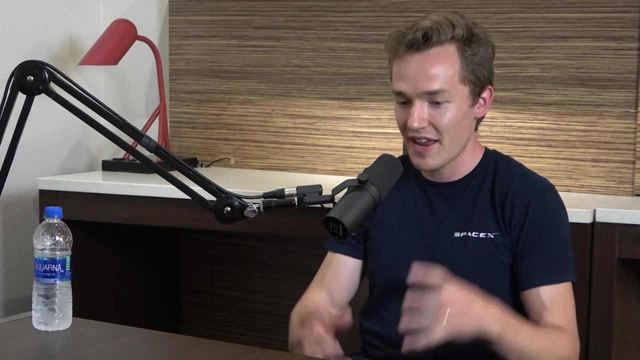 um, after you stir it and like, let's say, all the molecules settled to, like not moving again, one of the molecules will be basically in the same position it was before. Um, you have all sorts of fixed point theorems, like this right, That kind of fixed point theorem directly relevant to Nash. 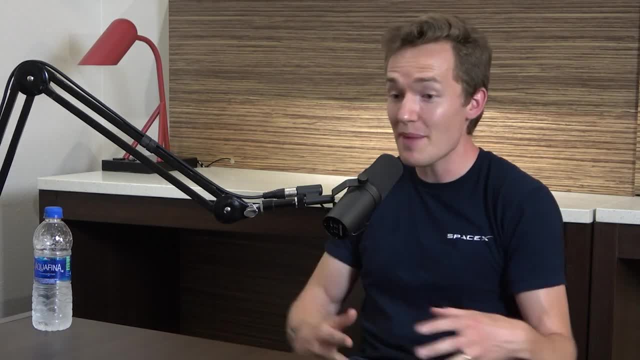 equilibriums, Right? Um, so you can imagine popularizing it by describing the coffee fact. but then you're left to wonder, like, who cares about if a molecule of coffee like stays in the same spot? Is this what we're paying?